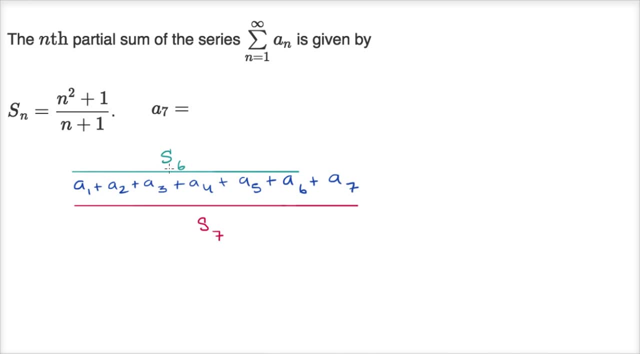 That's gonna be the sum of all of these, And then I can use that same formula to figure out the sum of the first six terms And the difference between the two. well, that's going to be r a sub seven. So another way of saying what I just said. 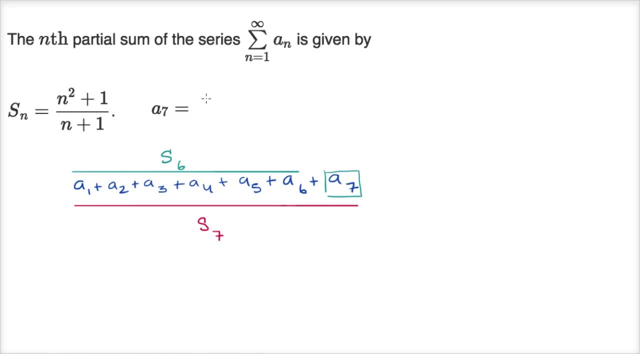 is that a sub seven is going to be the sum of the first seven terms minus the sum of the first six terms. Sum of the six: the sum of the first six terms. And if you were doing this problem on your own, you wouldn't have to write it out this way. 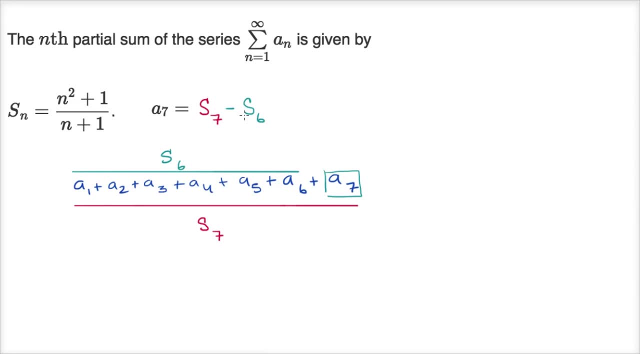 I just wrote it out this way, hopefully making this statement a little bit more intuitive: Well, what is, what are? what is this going to be? Well s sub seven, the sum of the first seven terms. we, just, wherever we see an n. 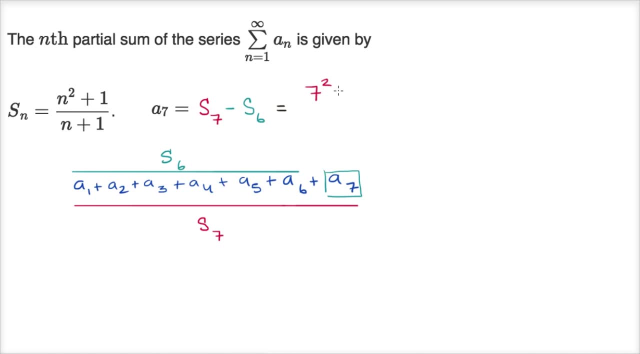 we replace it with a seven. So it's going to be seven squared plus one over seven plus one, And from that we are going to subtract s sub six, the sum of the first six terms. Well, that's going to be six squared plus one. 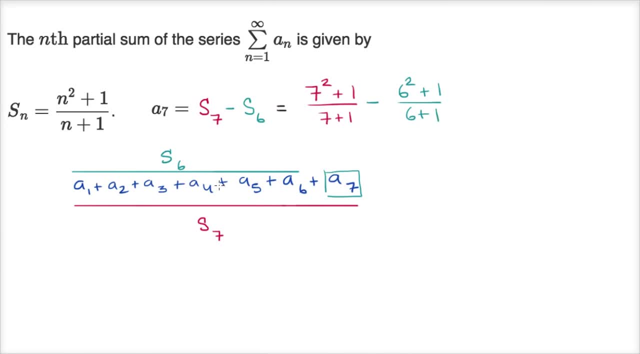 or six plus one, over six plus one, And from here we just have to do a little bit of arithmetic. So this is going to be, let's see, seven squared plus one. So this is 49 plus one, so that is 50 over eight. 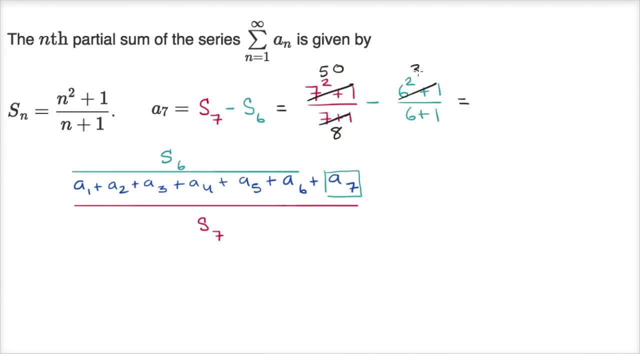 And this is six squared plus one that is 36 plus one that's 37, over seven. So let's see, we want to find a common denominator between eight and seven. That would be 56.. So this is going to be something over 56,. 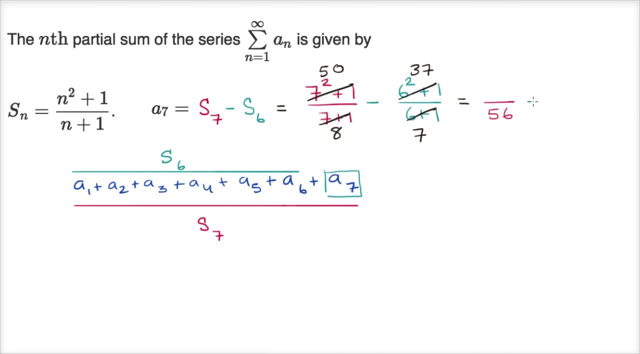 something over 56 minus something else over 56, minus something else over 56.. Now, to go from eight to 56, I multiply by seven, So I need to multiply the numerator by seven as well. 50 times seven is 350.. 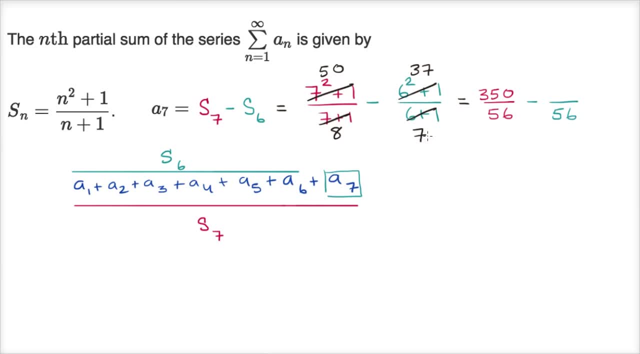 And then this second fraction. I multiply the denominator by eight to get to 56.. So I have to multiply 37 times eight And see: 37 times eight is going to be 240 plus 56. So that is 296, 296..